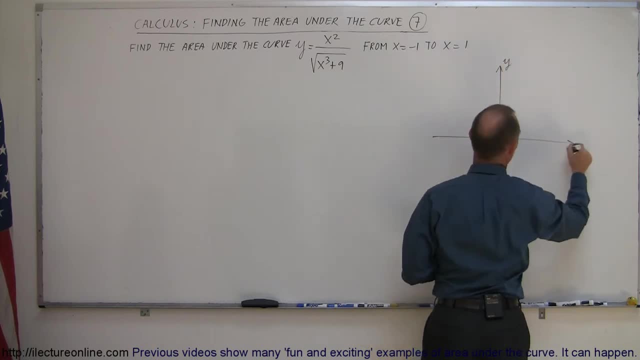 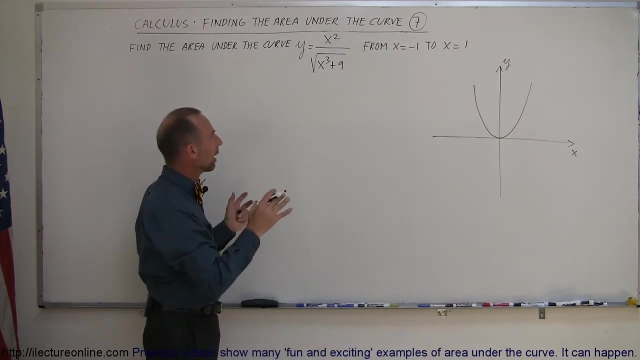 I will get the following: This is our y-axis, that's our x-axis. y equals x squared looks like something like this: It's a parabola opens upward, the vertex is at the origin. And then I'm going to graph just the denominator separately. So which is, let's say, y equals the square root of x cubed plus nine. And for the positive end of the spectrum, what do we get? Let's see here. So we probably 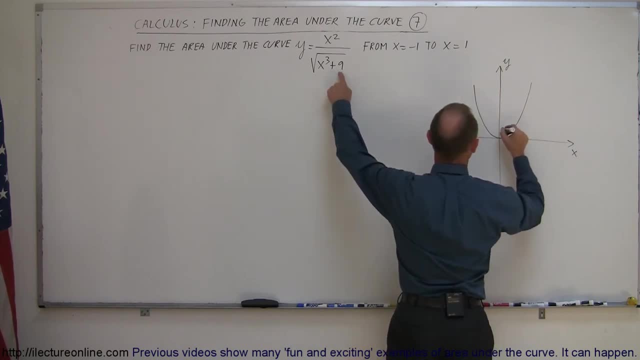 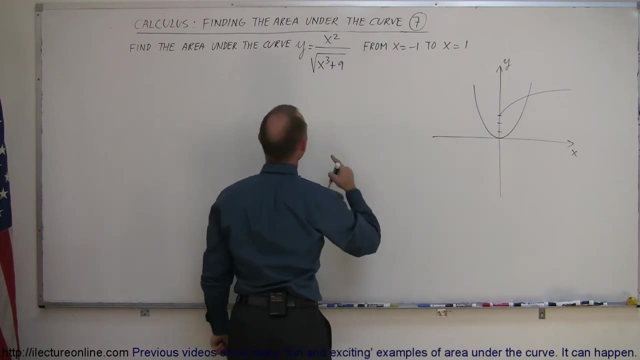 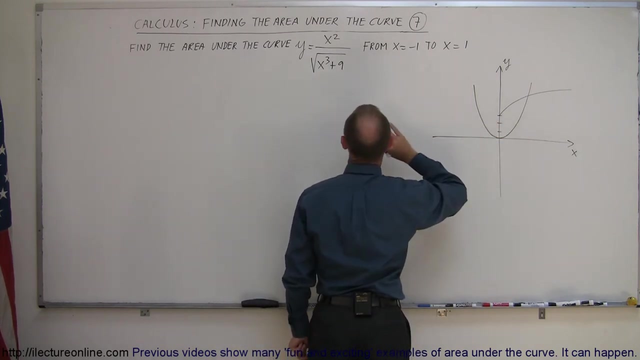 that's if x is equal to zero. the square root of nine is three. So one, two, three, And that probably looks like this on the positive side. Now the question is: can we have this on the negative side as well? Well, we can, to some. to an extent. we can let x be negative all the way out to almost minus two. So that means the equation can continue when x equals to minus two cube, minus 2.1 cube. So this continues on like this, And 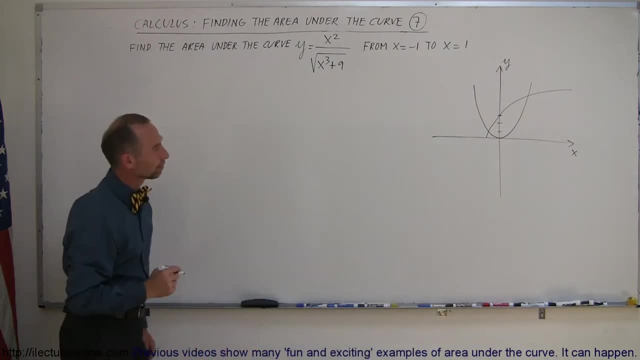 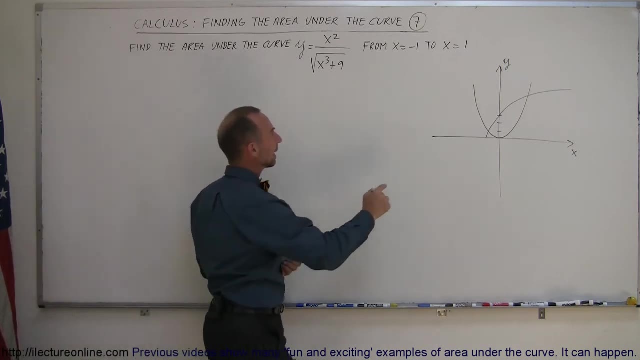 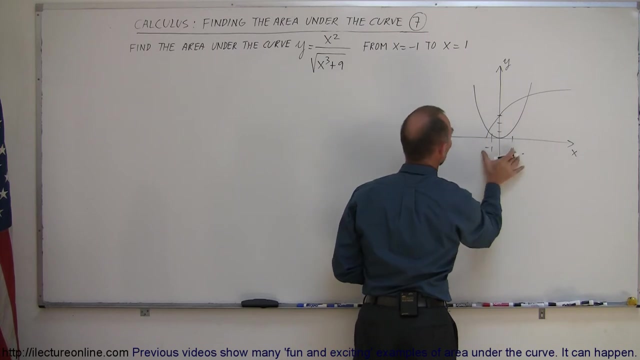 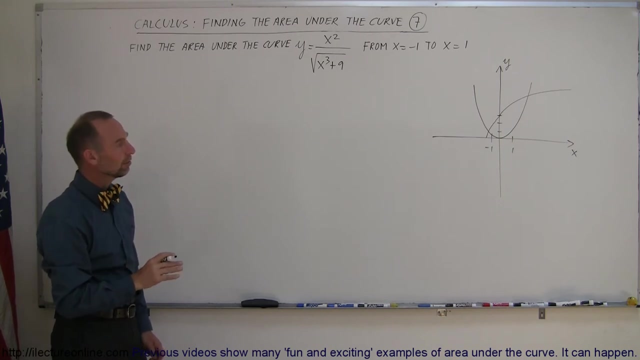 then we probably have to stop it because we cannot go negative on that. And so now we're trying to find the function where we take the x squared and divided by the denominator. But notice that for values from minus one to one- because those are the limits of my evaluation- both functions are either zero or positive, And the one that becomes zero is in the numerator, So I don't have to worry about that. That means when I divide, 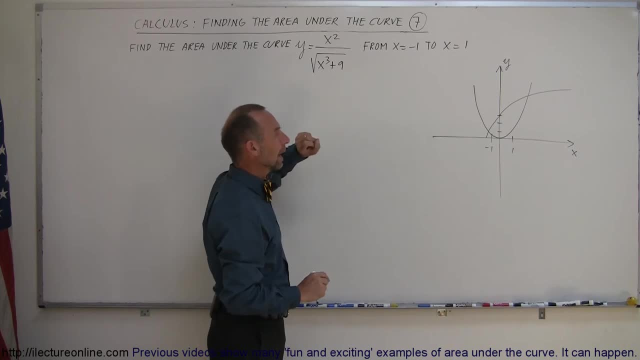 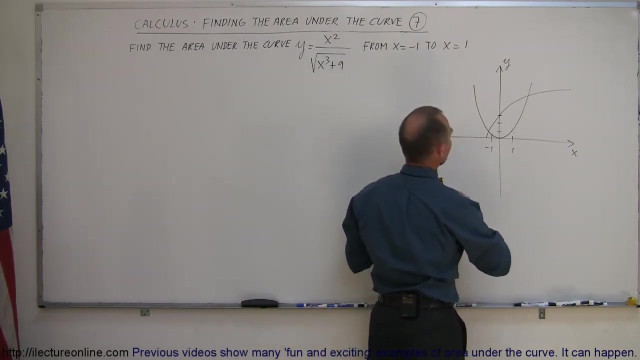 the x squared by the square root of x, cube plus nine, I will get a positive value In the case. of course over here we get a zero, but I don't worry about that And that means that whatever the function is, it looks like. if I were to guess what that function looks like, it probably looks something like this: Let's see here something like this, And then it comes up and it probably looks something like that. So it looks like I can find the area and need this curve. 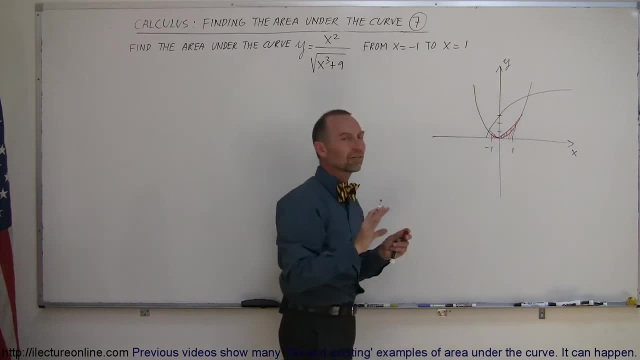 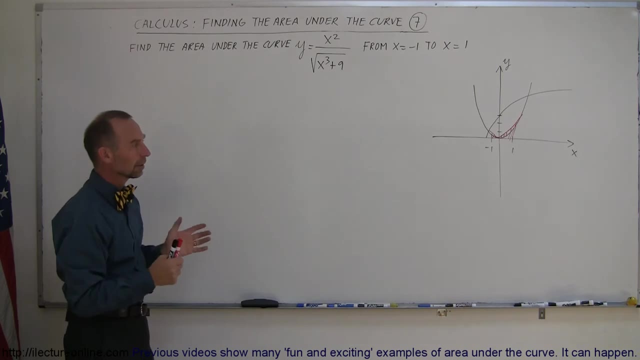 It'll probably look something like that. So it's a rough approximation of what that curve looks like when I divide the numerator by the denominator. I just want to make sure that it doesn't go negative anywhere, and it looks like it does not. Okay, I'm now ready to go. So let's say that the area then is equal to the integral from x equals negative one to x equals positive one of the value of x squared divided by the square root of x cube plus nine. 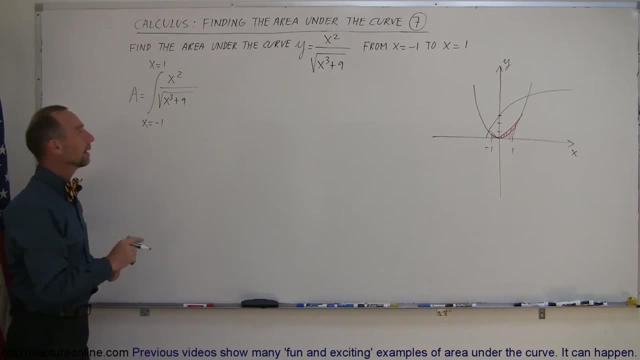 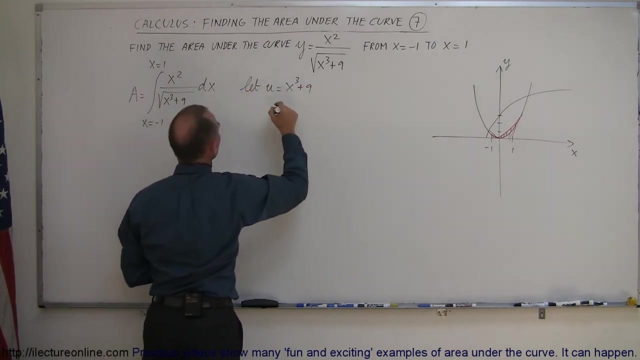 Hey, it looks like that. Oh, and don't forget my dx. Now it looks like the x squared is a derivative of the x cube underneath the radical. That gives me an idea. I'm going to let u equal x cube plus nine. Then my du dx is going to be equal to three x squared and the nine. of course that's a zero, And so du is equal to three x squared dx. 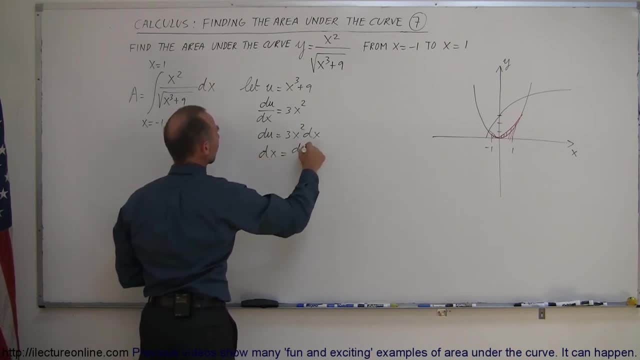 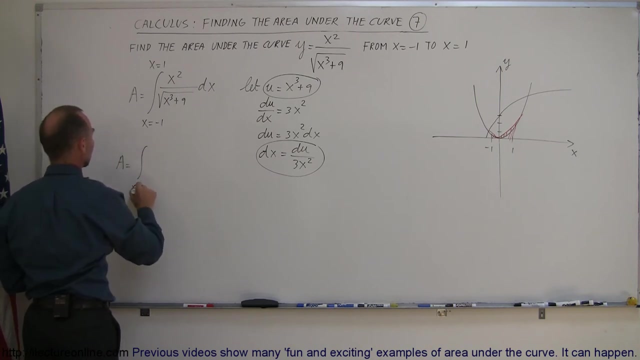 Or the x is equal to du divided by three x squared. All right, I'm now ready to substitute this and this into my integral. When I do that, I get the following: I have a. the area is equal to the integral from x equals negative one to x equals one. The denominator stays there, That's x squared. The denominator would be the square root of this quantity right here, which is equal to u. 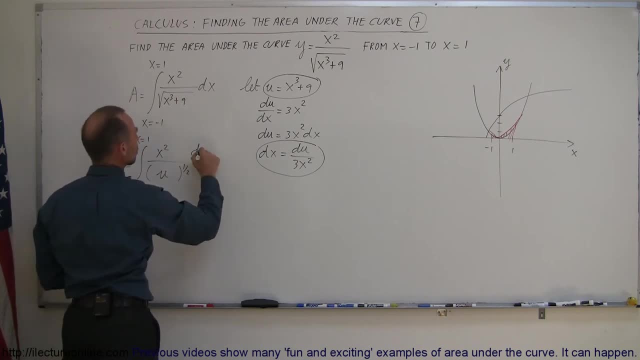 And instead of dx I'm going to write du divided by three, x squared. Okay, the next thing I can do now is notice that this x squared will cancel out that x squared, So I don't want to have any x's inside my integral. The one over three can be taken out, And so I can now write this: as the area is equal to one over three times the integral from x equals negative one to x equals one of one over u to the one half du, which, of course, I can write as the area. 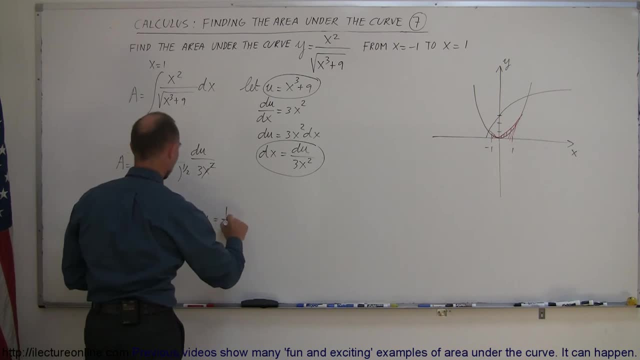 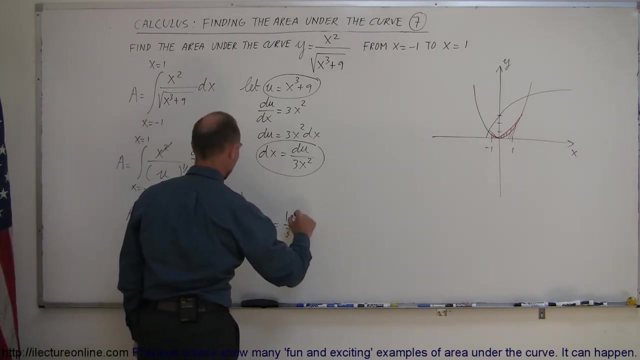 I'm going to bring to the numerator and turn it into a negative exponent. So this is equal to one over three times the integral from x equals negative. one to x equals one of u to the minus one half du. And now I'm ready to integrate that The integral of that is one third times. that would be u to the one half power, because I add one to the exponent divide by the new exponent one half, and then I have to evaluate that from x equals negative, one to x equals one. 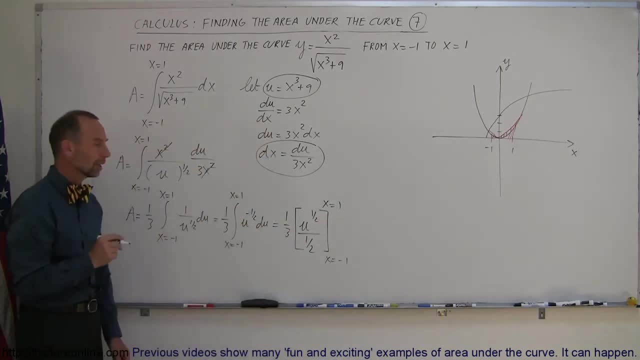 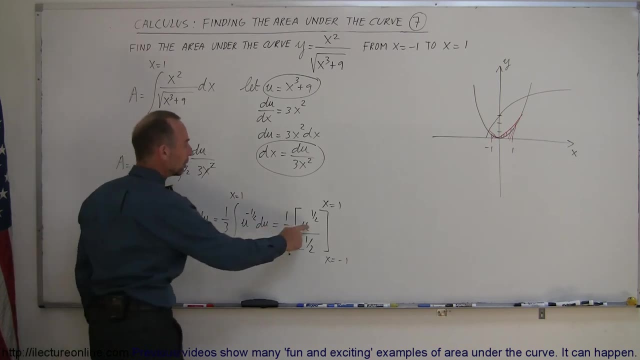 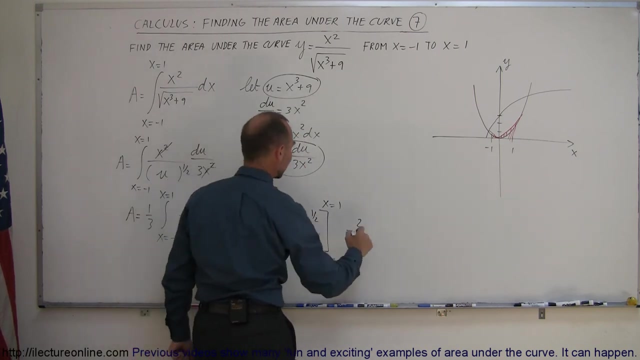 So that's why I keep putting in the variables for the limits, to show you that the limit variables are not the same as the variable here. So I first have to convert that back to the x variable. Okay, anyway, one third divided by one half. When you divide by a fraction, the same is multiplying by its inverse, So this becomes two thirds. Instead of u to the one half, I'm going to write x cubed plus nine to the one half power, So this becomes x cubed plus nine to the one half power. 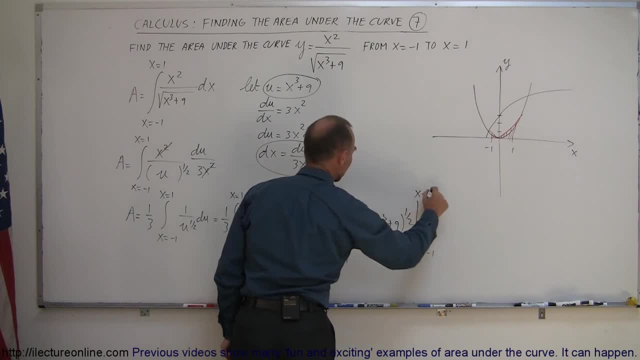 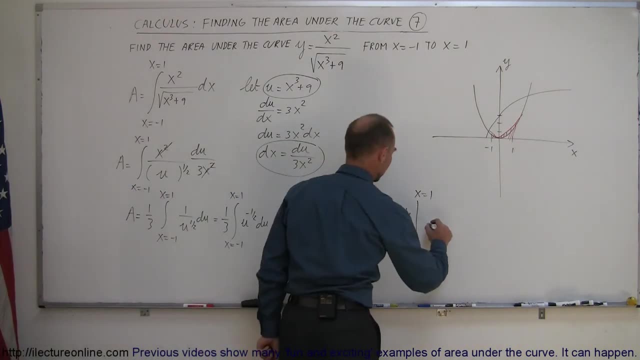 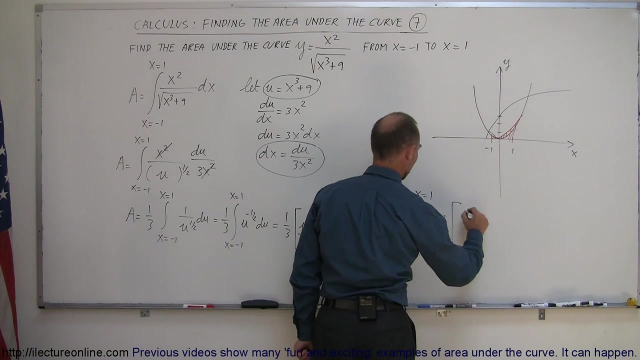 and evaluate it from x equals negative 1 to x equals 1.. And now I'm ready to go ahead and plug in the values. Okay, this is equal to 2 thirds times. when I plug in the upper limit, I get 1 cubed plus 9,, 1 cubed plus 9, raised to the 1 half power. 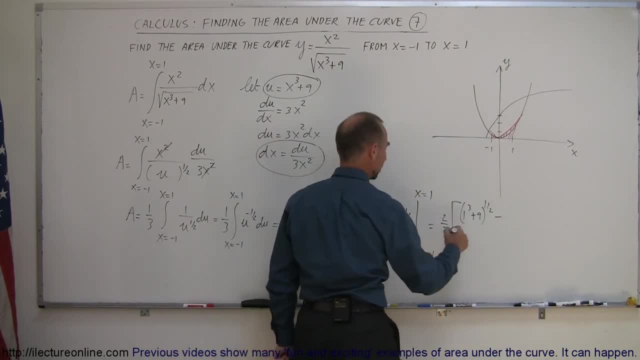 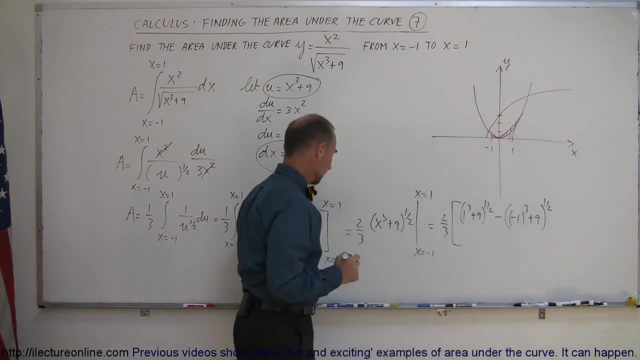 Then I subtract from that. when I plug in the lower limit, That would be minus 1 cubed plus 9 to the 1 half power, And I guess that's it, The 2 thirds. I factored it out, so I can leave it like this. 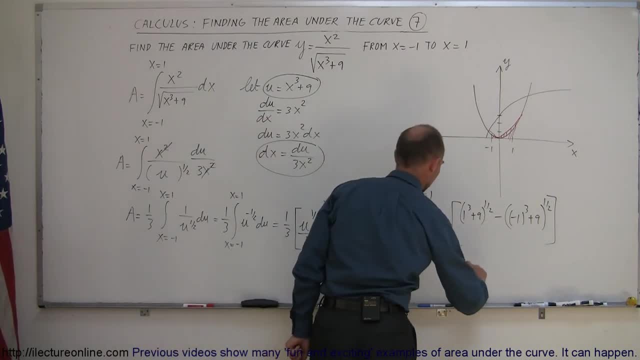 Which means this is equal to 2 thirds times 1 plus 9 is 10, so that would be the square root of 10.. That would be 10 to the 1 half power Minus. this is minus 1 plus 9, that would be 8.. 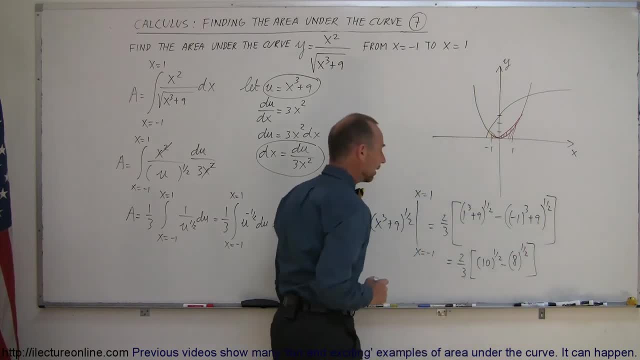 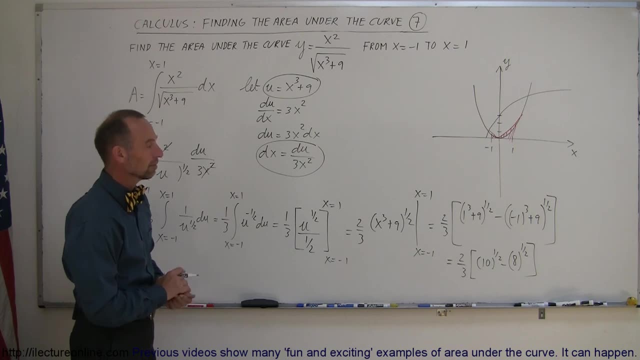 To the 1 half power, And I guess we could simplify that any further, but that's good enough. So 2 thirds times the square root of 10 minus the square root of 8. And I'll go ahead and leave it like that, even though I can simplify it just slightly more.